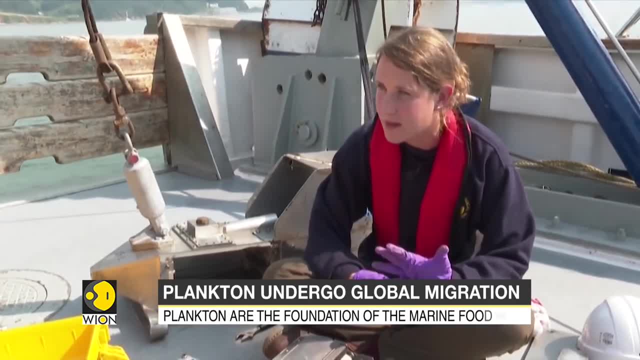 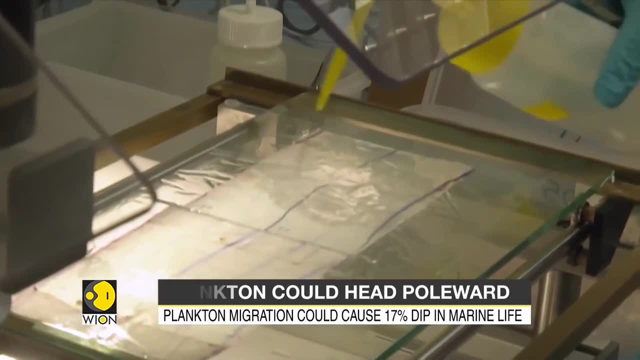 How that's impacting food webs, which new species are coming into the area. So these are the kind of key things that we're looking at. Back on dry land, scientists look through the samples and identify the different species of plankton they collected. 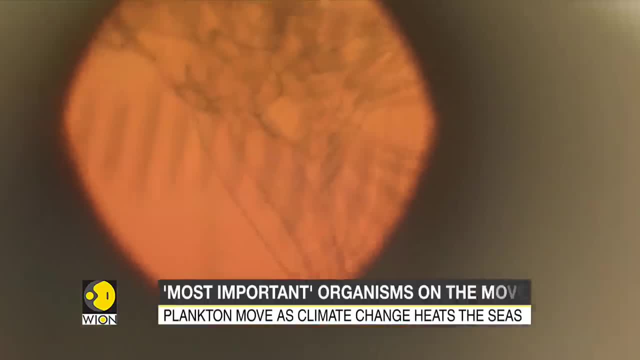 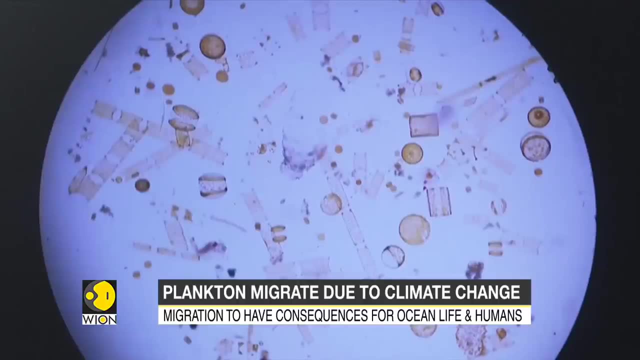 There are two main types: phytoplankton- diverse plant-like cells, commonly called algae, and zooplankton- animals like krill and the larvae of fish, crabs and other marine creatures. Both are crucial players in the ocean's development. 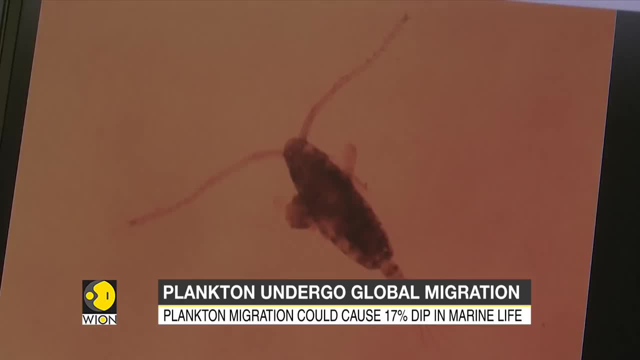 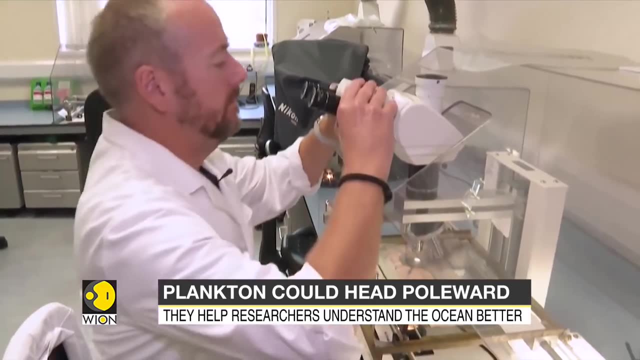 Subtitles by the Amaraorg community food chain. but phytoplankton are also behind nearly half of the world's oxygen and help trap at least a quarter of CO2 emitted by burning fossil fuels. But like many marine animals, plankton have been on the move, heading for cooler areas. 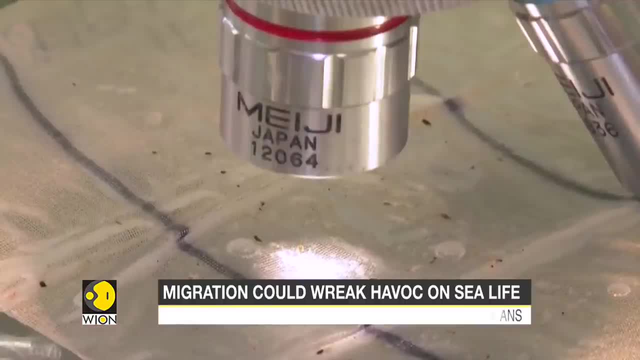 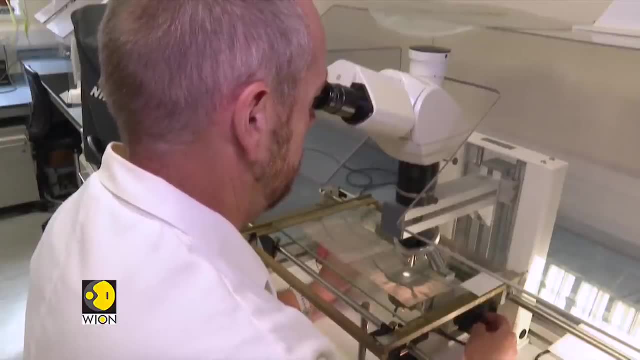 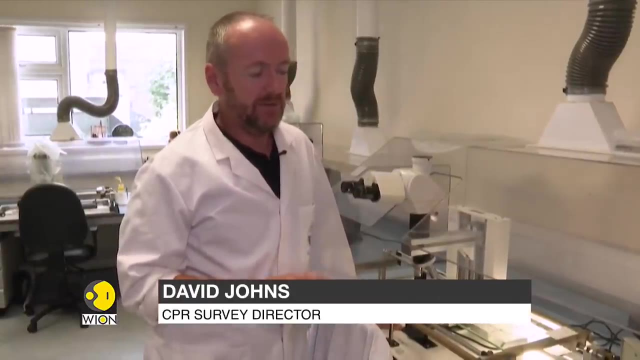 like the Earth's poles, Smaller warm-water plankton are also replacing the more nutritious cold-water ones, meaning the species that feed on them need to adapt or move too. If we think about global warming and a warming ocean, we've seen that that can have direct, rapid responses on the plankton. 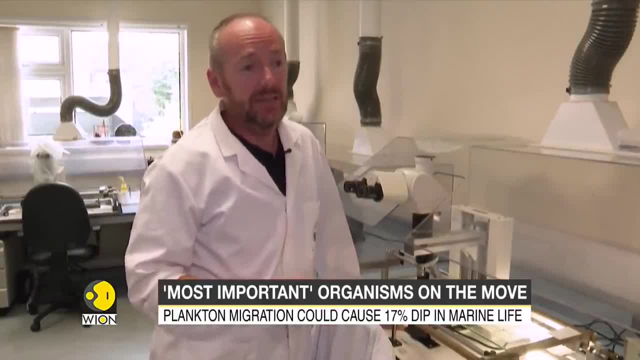 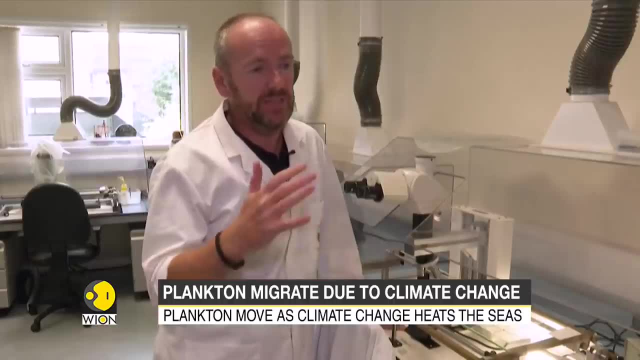 particularly the zooplankton, causing them to change in their seasonality, causing them to change in their nutritional quality and the areas where you find them. So we're tending to find that they're shifting out of their normal ranges, which then has. 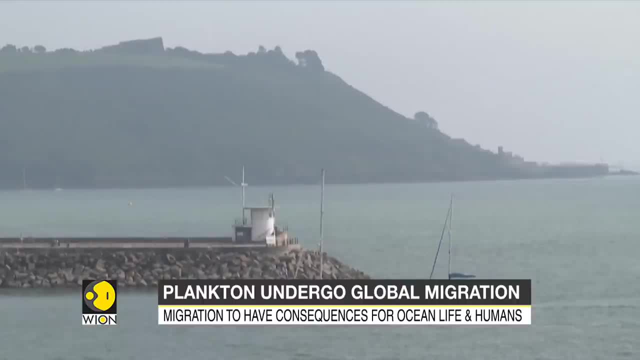 an impact on fish that like to eat them. According to a leaked report by the UN's Intergovernmental Panel on Climate Change, due to be published next year, the total quantity of phytoplankton that are found in zooplankton. are more than half of the total amount of phytoplankton that are found in zooplankton. According to a leaked report by the UN's Intergovernmental Panel on Climate Change, due to be published next year, the total quantity of phytoplankton that are found in zooplankton are more than. 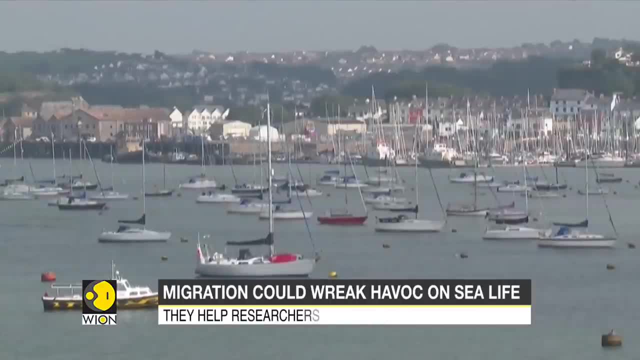 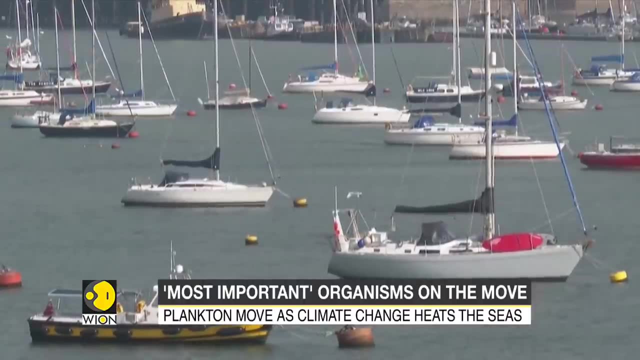 half of the total amount of phytoplankton that are found in zooplankton. Phytoplankton is predicted to fall by around 1.8 to 6% over the next century, depending on greenhouse gas emissions. Because of plankton's outsized importance, even such modest reductions could mean an 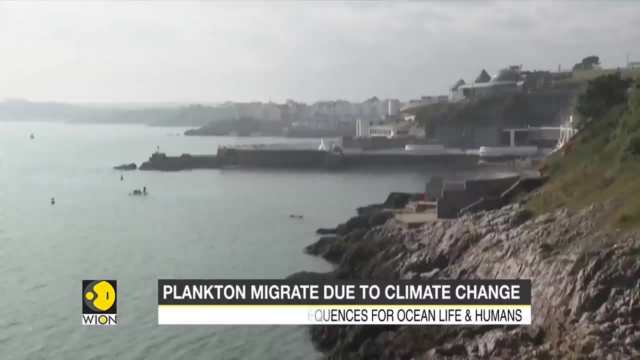 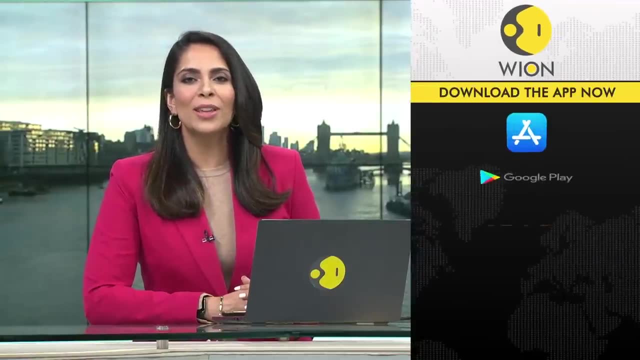 eventual loss of up to 17% of marine life.